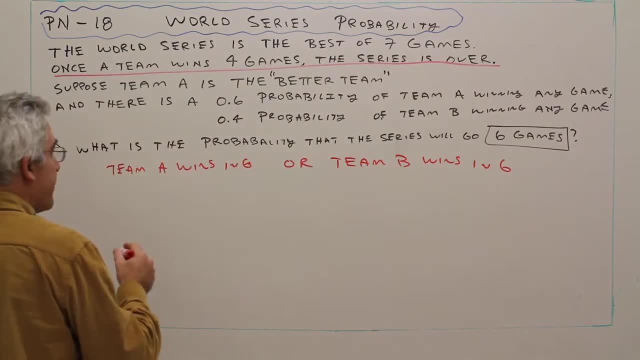 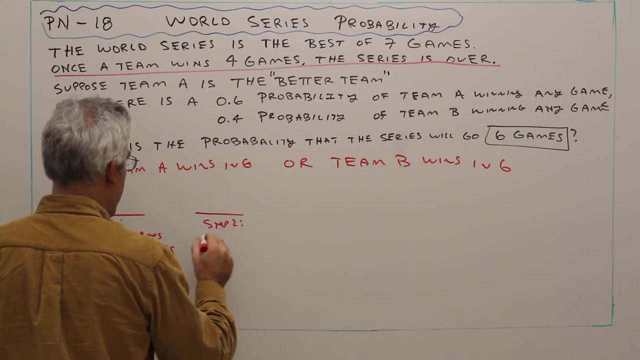 and then Team B has won the sixth. All right, so let's set that up. All right, so two steps. Step one, so it's gone to five games. Basically, A has won three games, B has won two games. So the number of ways of doing that. and then step two. 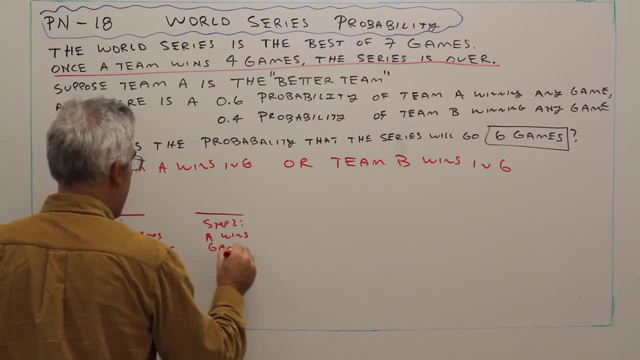 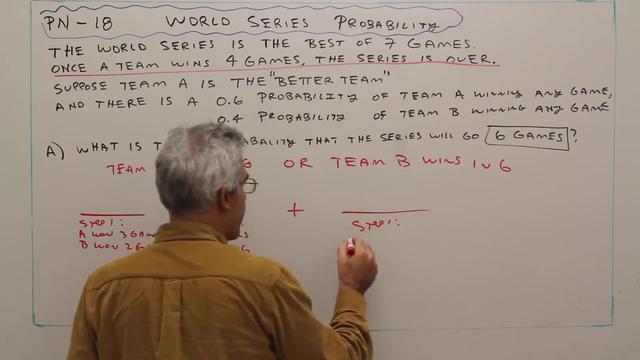 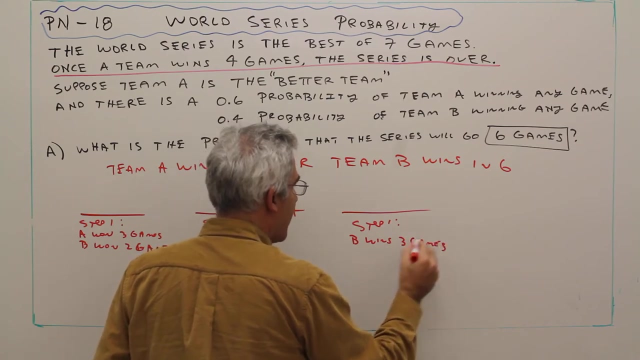 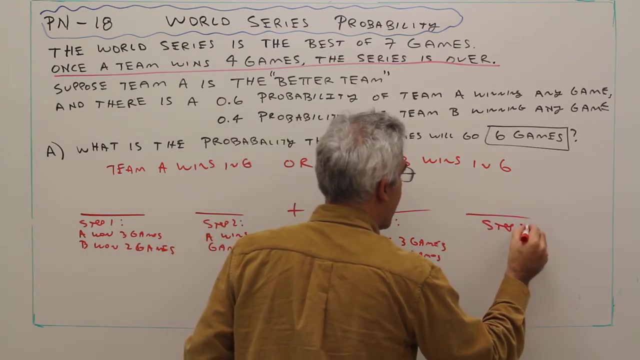 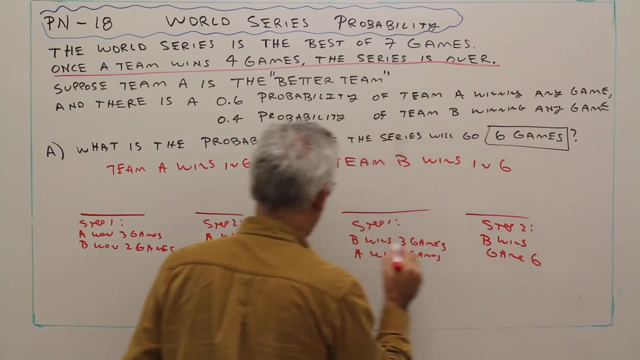 A wins game six. Likewise over here, step one, in this case B wins three games. A wins three games. A wins three games, B wins two games. And then step two: B wins game six. Okay, so what I've got to do is find the probability. 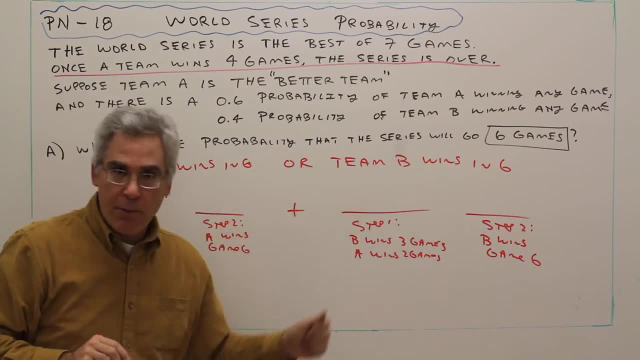 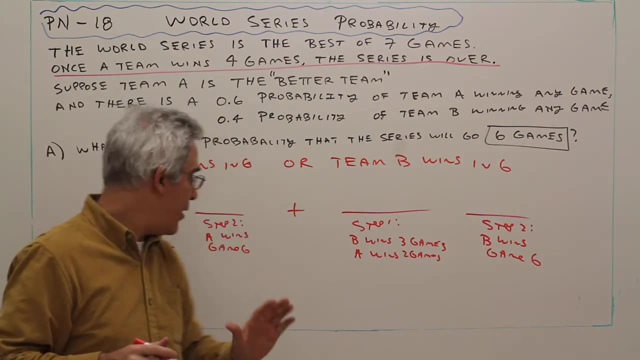 of each step. multiply it, add it over there and I'm done. Okay, so I've got five games that have been played And A has to have won any games. A has won any three of those. So just to give you a visual: 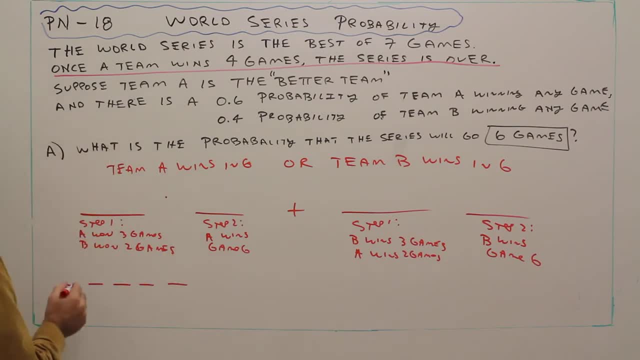 So out of five games, A has won three, For example. it could be A A, A, B, B, et cetera. It could be A A, B, A B, So the number of ways that can happen is out. 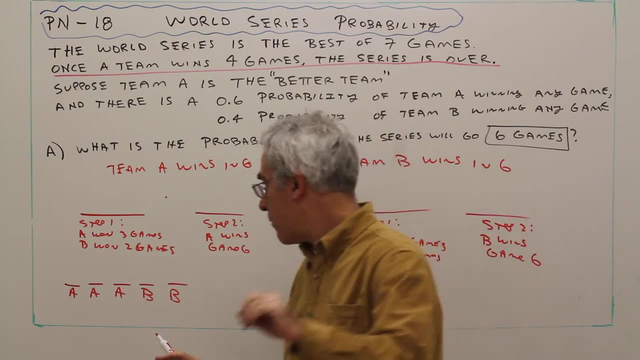 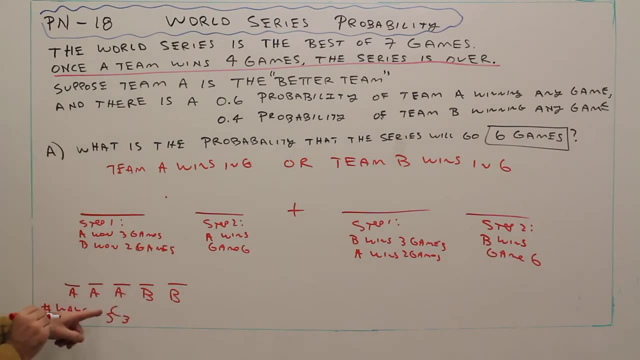 of five slots, choose three of them for A to have wins. So the number of ways that can happen It's 5, choose 3.. And then, for each one of those branches, the probability is 0.6,, 0.6, 0.6,. 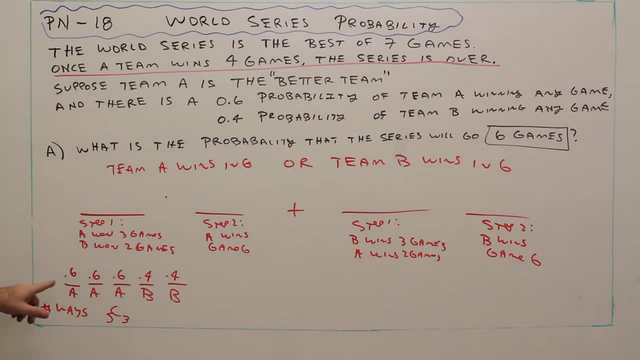 0.4, 0.4.. So pretty much for this step right here. I'll do it in black. there's going to be 5: choose 3 times 0.6, cubed, times 0.4 squared. That's just for it to get to that point, And then, if A wins, 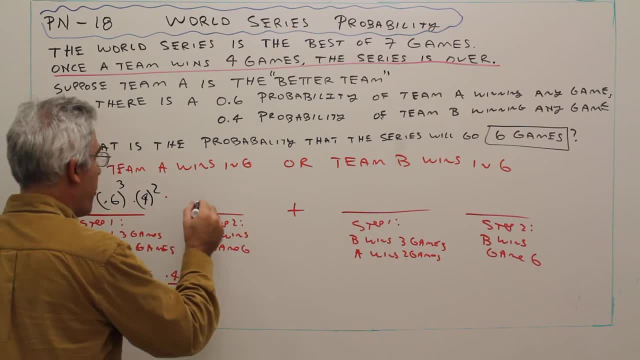 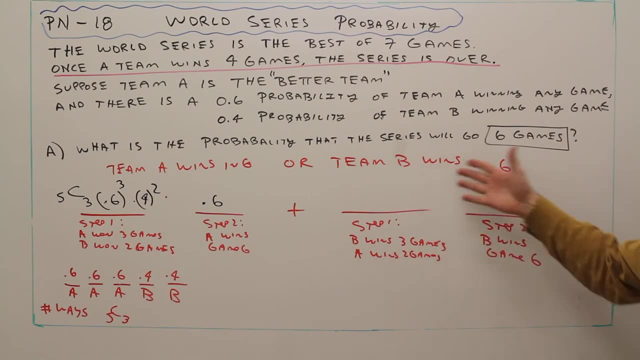 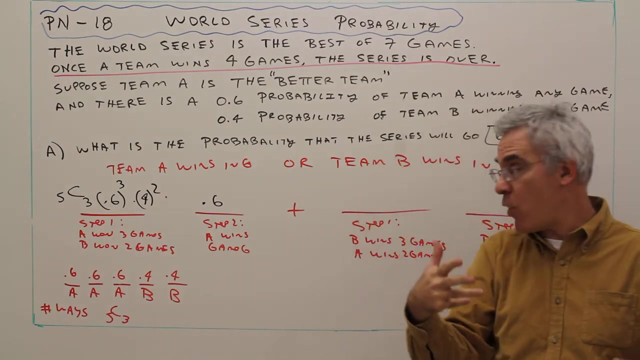 game 6,. well, the probability of that happening is just one more 0.6.. Okay, let's do it over here for team B. This is for team B winning in 6 games. Again, it must have gone to 5 games and B must have won 3 of those 5.. 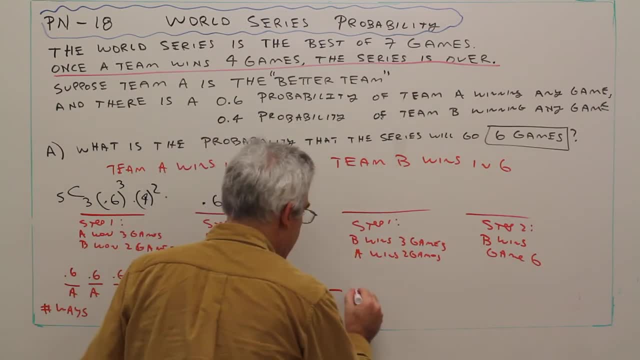 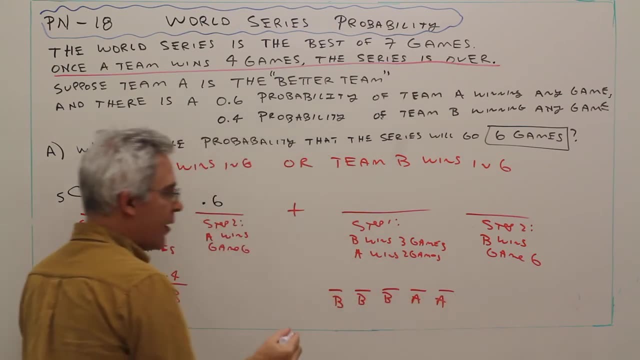 So I'll just set it up like this: 1, 2,, 3,, 4,, 5.. So, for example, it could have been B, B, B, A, A- Again there's 5. choose 3 ways. 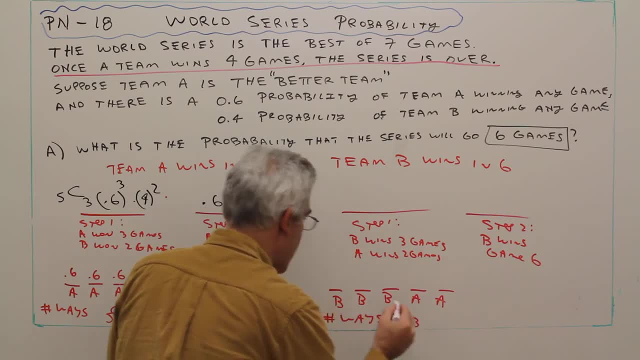 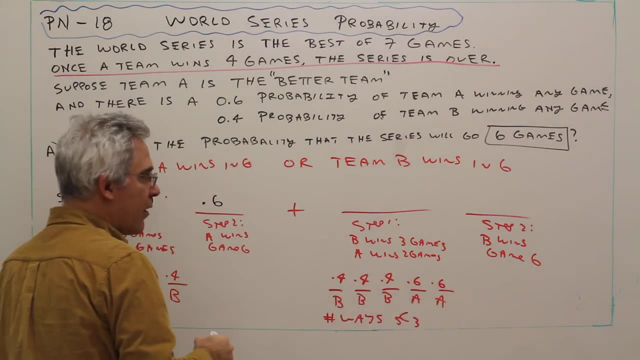 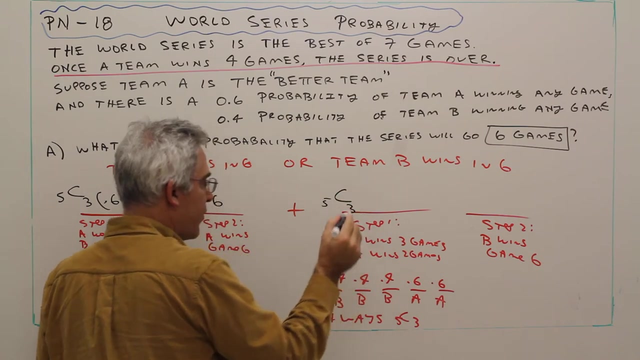 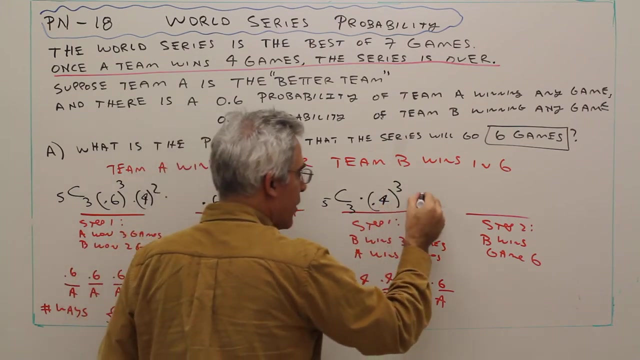 And the probabilities are 0.4, 0.4, 0.4, 0.6, 0.6.. So the probability of that step is going to be 5. choose 3 times 0.4 cubed. 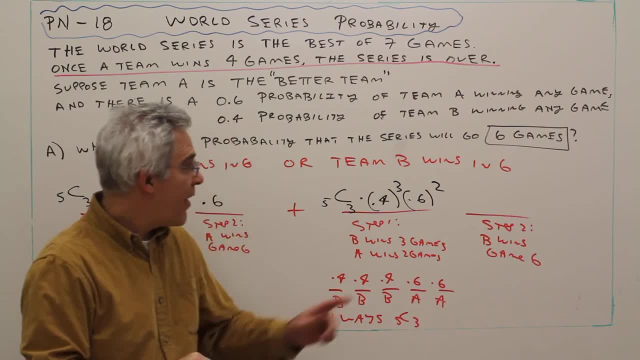 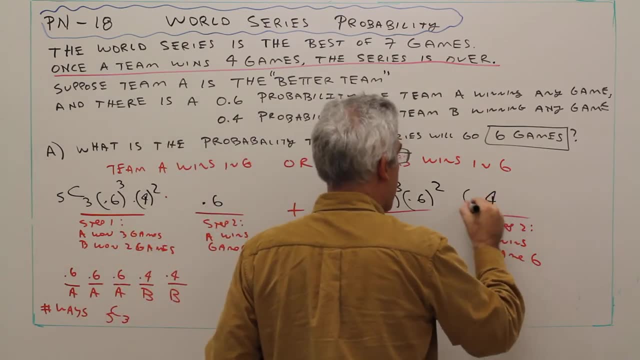 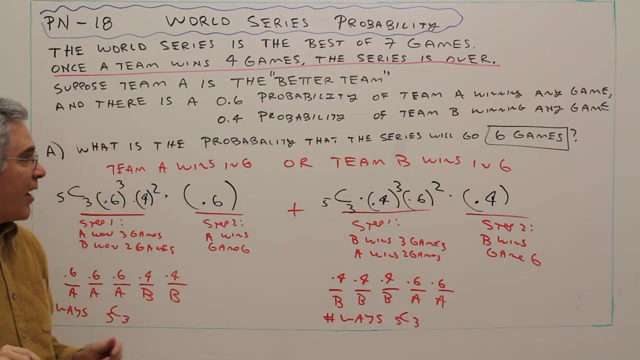 times 0.6 squared. And then again B is winning the 6th game. The probability of B winning any game is 0.4.. And just so you know, I'm multiplying And that's the setup. To save time, I've 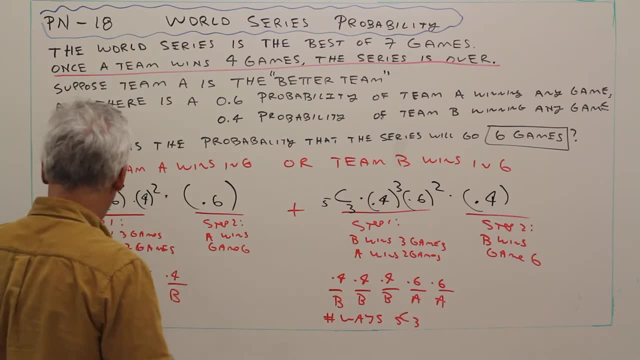 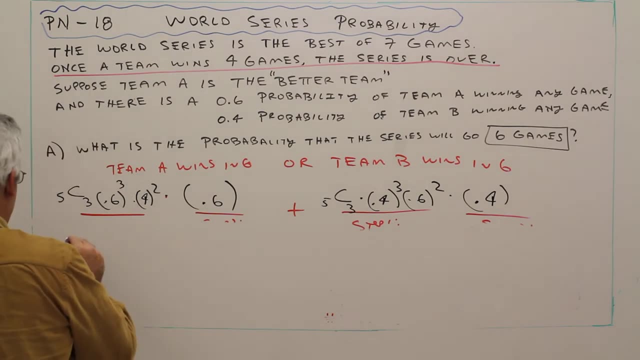 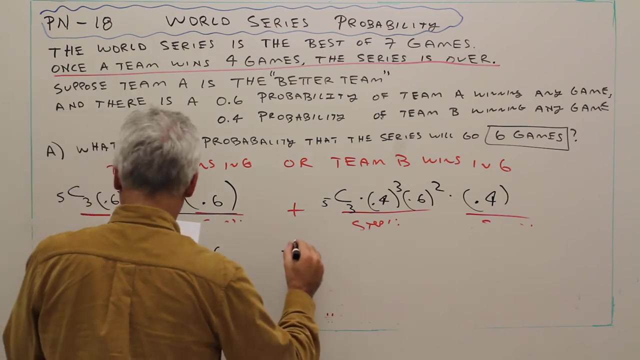 computed it already, So let me just erase this. I got 10, that's for that times. all of this was 0.0,. I'll just write down the final answers. This was 0.20736 plus 0.09216. 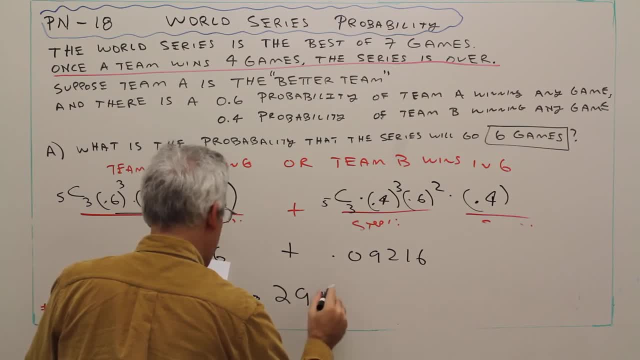 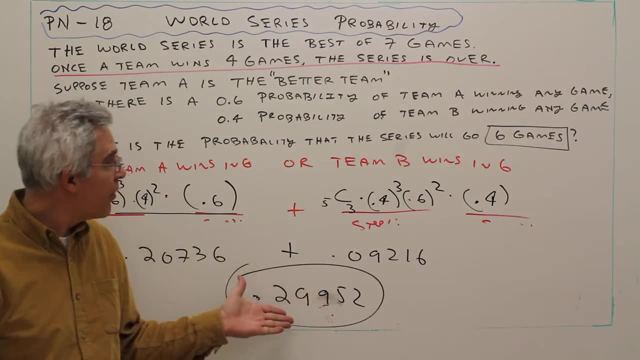 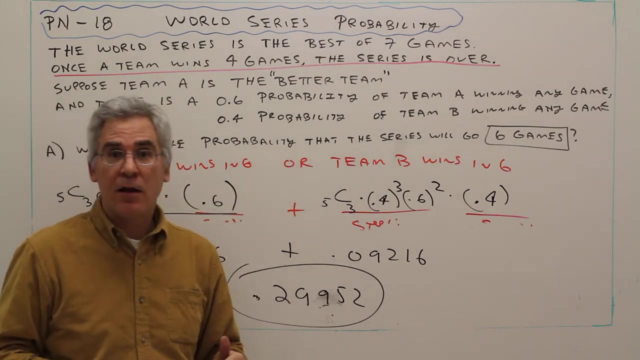 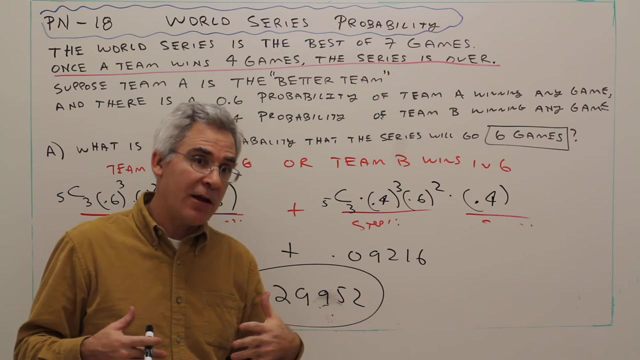 for a sum of 0.29952.. And that's the answer for, in this situation, the probability that the World Series will end in exactly 6 games. Part B is going to be the probability that it will end in exactly 7 games, And I encourage you to try to work it out. 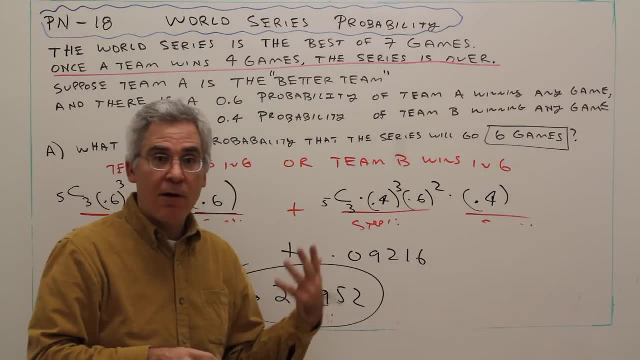 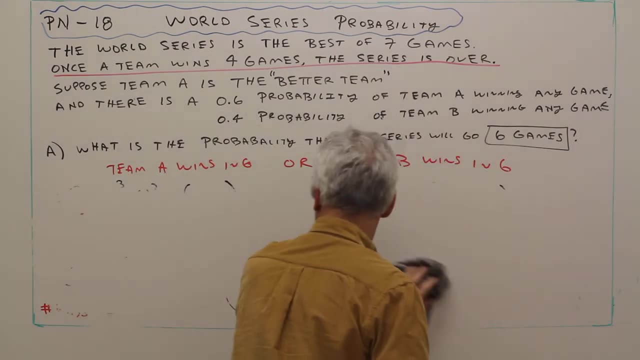 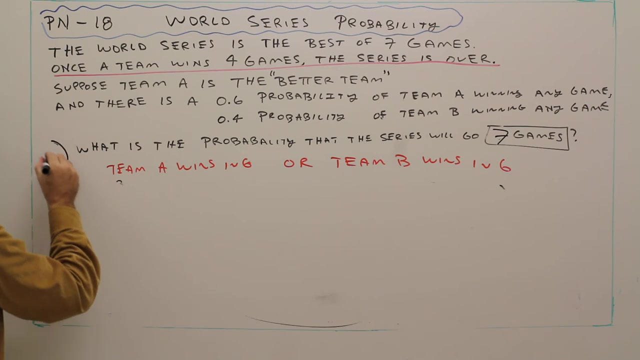 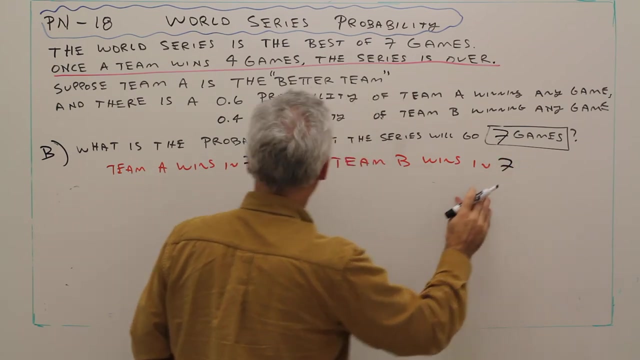 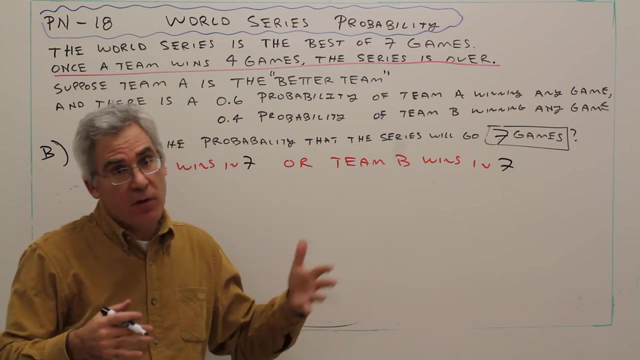 on your own first And then, if you have questions, follow along with my solution. So here I go with Part B. Okay, so Team A could win in 7 games or Team B could win in 7 games. It's going to be a similar setup. 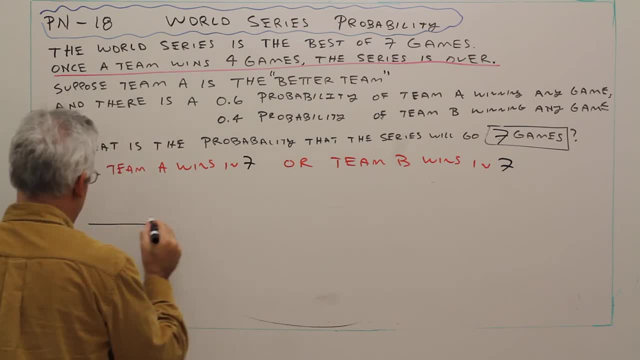 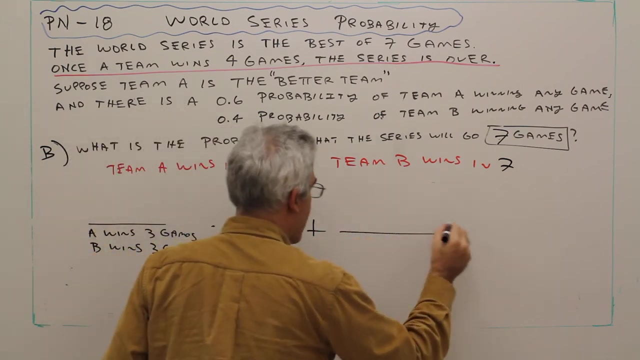 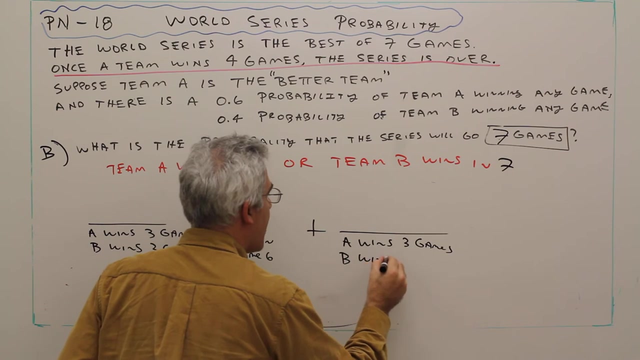 So let's see if we can do it a little bit quicker. So the first step is: A wins 3 games, B wins 3 games, Times A winning in game 6.. Plus, again, A wins 3 games, B wins 3 games. 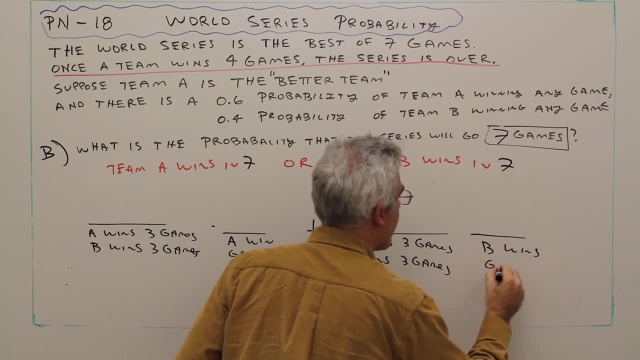 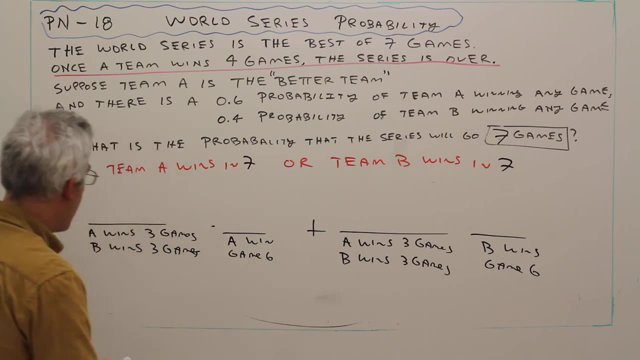 And then B wins in game 6.. Okay, So let's see if I can do this. So the number of ways that this can happen is: I have 6 games. Choose 3 of them for A to win, So 6, choose 3.. 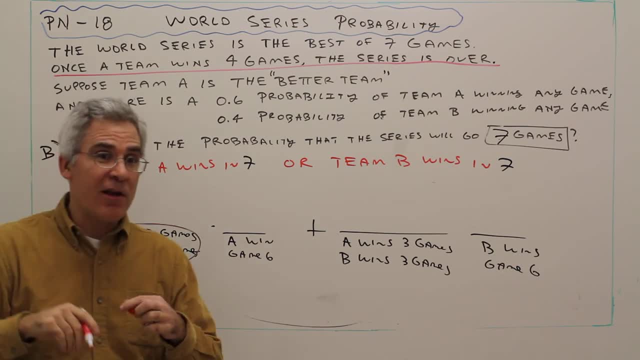 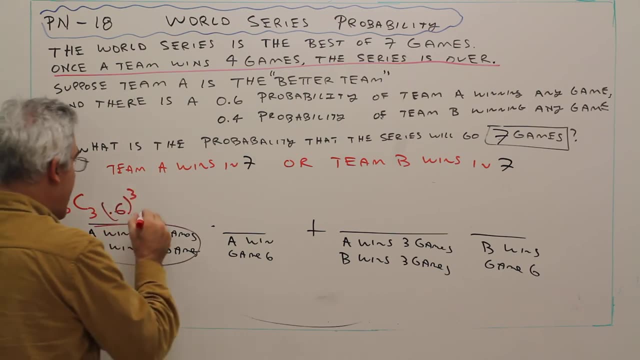 That'll take care of that. And then the probability of each step is: Oh, if A's winning 3, that's 0.6 cubed. If B's winning 3, that's 0.4 cubed. If A is winning in that. 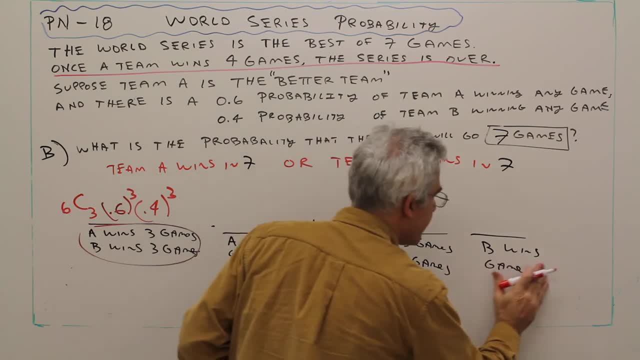 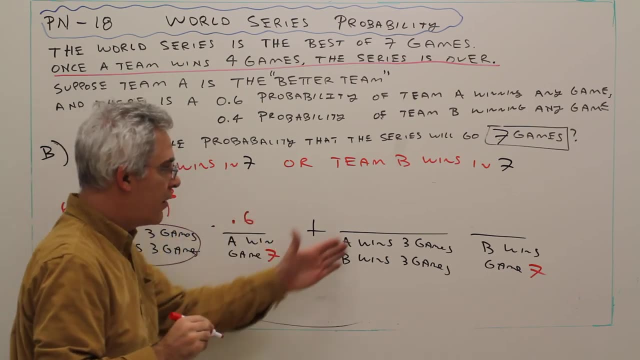 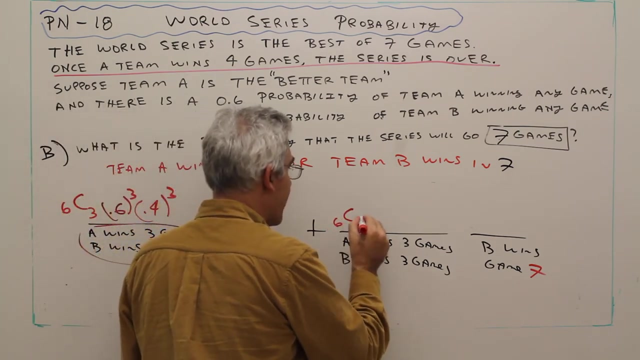 Ooh, This is game 7.. Sorry about that. If A wins in game 7, well, that's just 0.6.. Okay, now for B winning in the 7th game. Again, there's 6.. 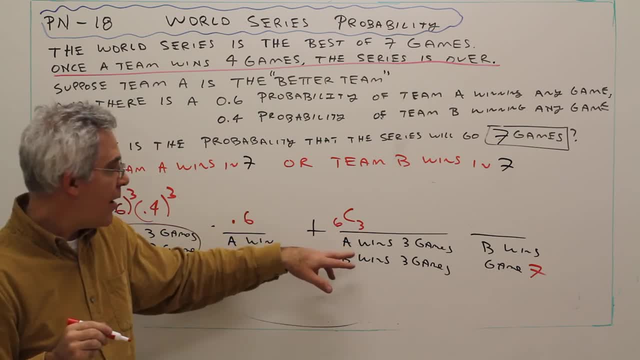 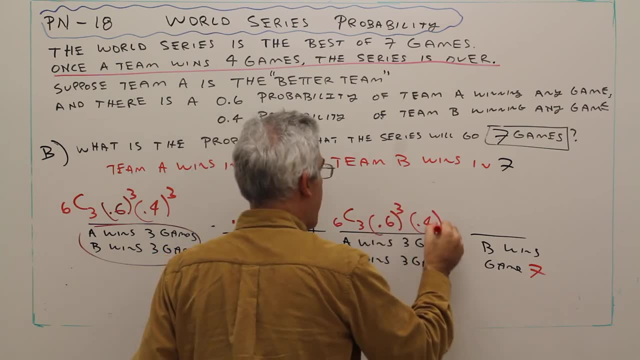 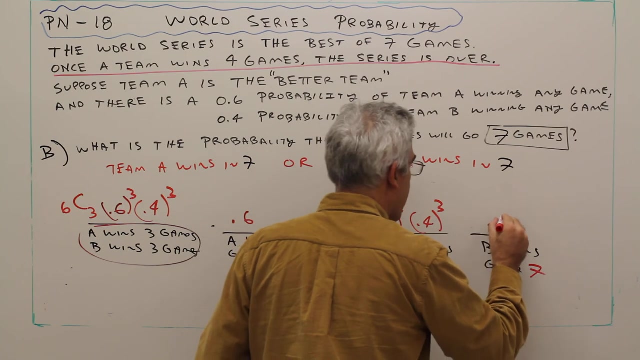 Choose 3 ways for that to happen. Again, it's going to be the same. I'll just do it the same: 0.6 cubed- 0.4 cubed. Now B is winning in game 7, so it's going to be a 0.4..